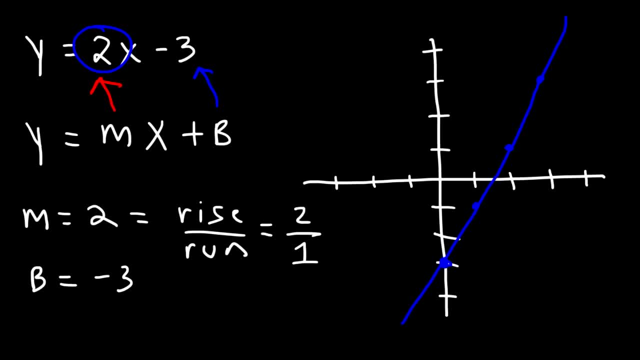 do is connect the dots with a line, And so that's how you can graph a linear equation in slope intercept form. Now let's try another example. So let's say we have the equation y is equal to three x minus four. Based on a previous example, feel free to pause the video. 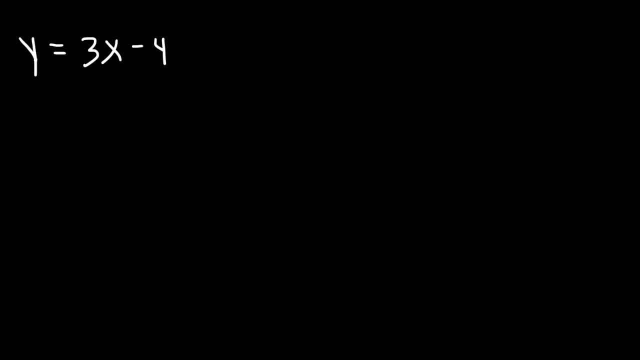 and work on this problem. Go ahead and graph that linear equation. So first we need to draw a graph. Let's put a graph here, Let's put a graph here, Let's place the marks on the graph. So while I'm doing this, you can graph the function. 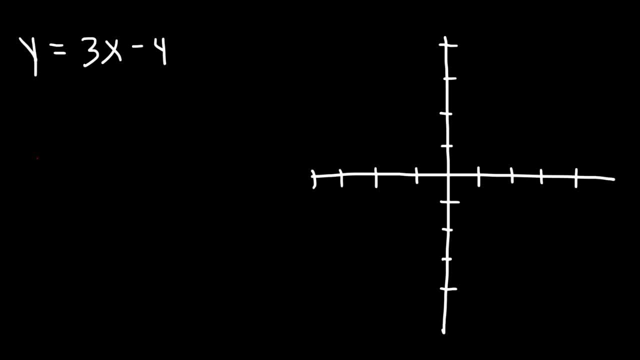 Now, what is the slope and y-intercept in this equation? So remember the slope-intercept. formula y is equal to mx plus b. The slope is m, which is the number in front of x, So the slope is three. 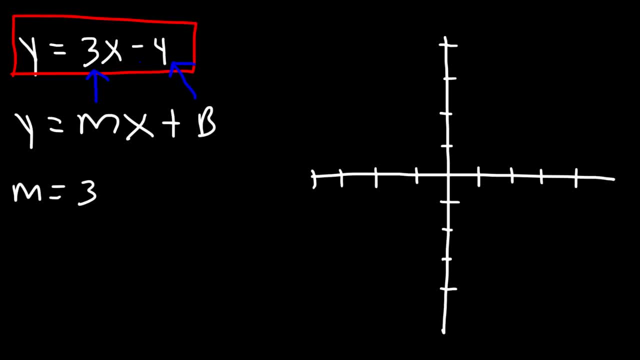 The y-intercept is b, which is the constant value at the end, And that's negative four. Now let's start by plotting the y-intercept. So it's negative four along the y-axis. So this is negative one, negative two, negative three and negative four. 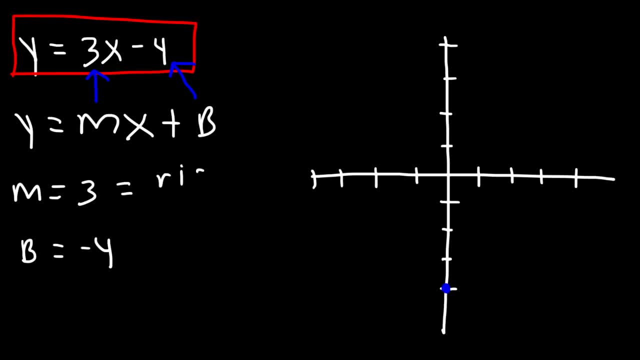 Next let's use a slope. The slope is the rise over the run, So a slope of three, or it's the same as three over one. So we have a rise of three and a run of one. So, starting from the y-intercept, we're going to rise or go up three units for every one unit. we 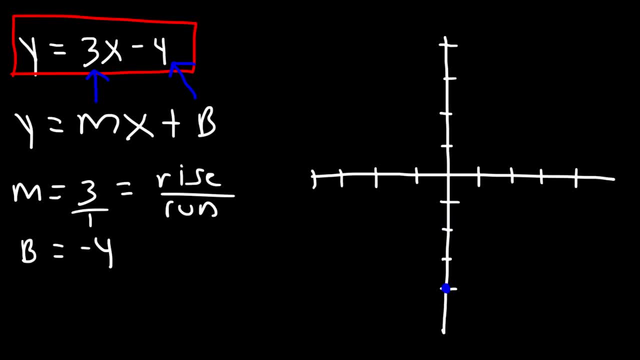 travel to the right. So that's the slope of three. Now, starting from the second point, we're going to travel up three units And then one unit to the right. So we have the point two comma two, And we could do it one more time: Go up three and then over one. 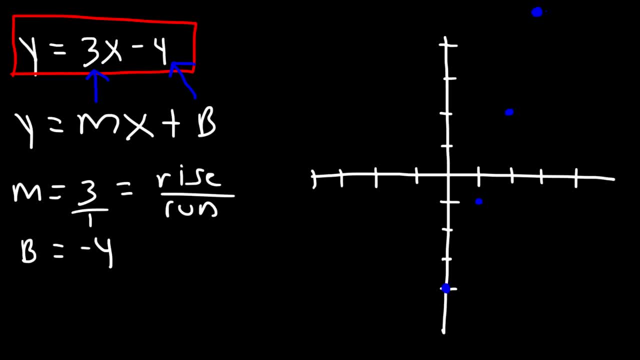 But we really don't need to. So that's going to be approximately somewhere in that region, But now we have enough information to draw a graph. My graph is not perfectly straight, but the idea is that you can use a rule if you want. 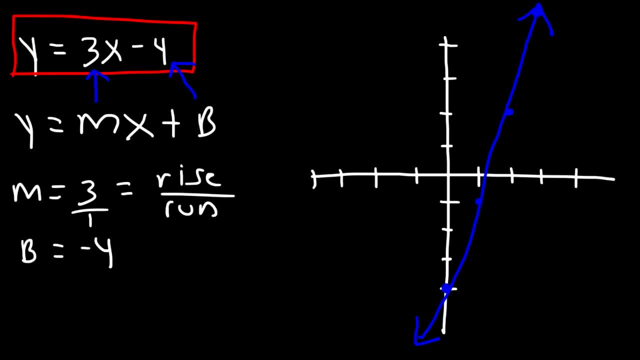 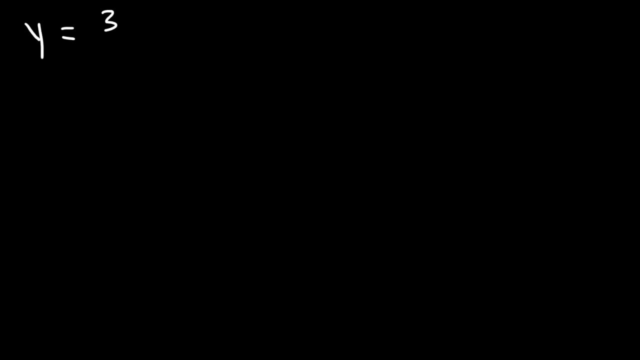 You just need to draw a straight line through those points, And really all you need is two points to draw a linear function. So the last two points really wasn't necessary. Now let's work on another example, By the way, for those of you who want more practice on graph and functions, 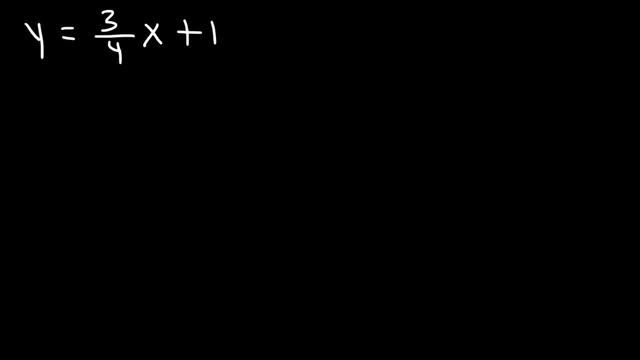 and not just linear functions. check out the description section of this video. I'm going to put some links to some other videos in that area, So if you're interested, feel free to check out my other videos on this. Thank you, See you next time. Bye. 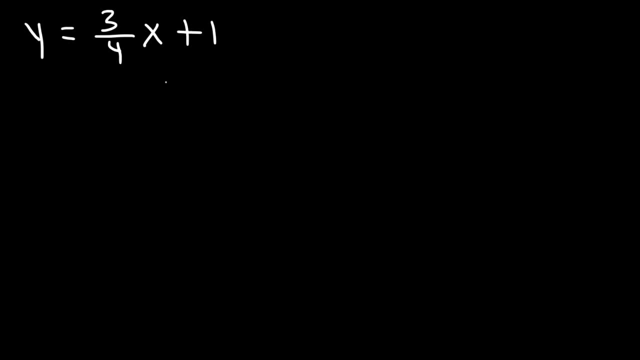 feel free to take a look at that when you get a chance. now, what if we have a fractional slope? what should we do in this example? so we have a slope of 3 over 4 and a y-intercept of 1, so go ahead and graph this particular function. 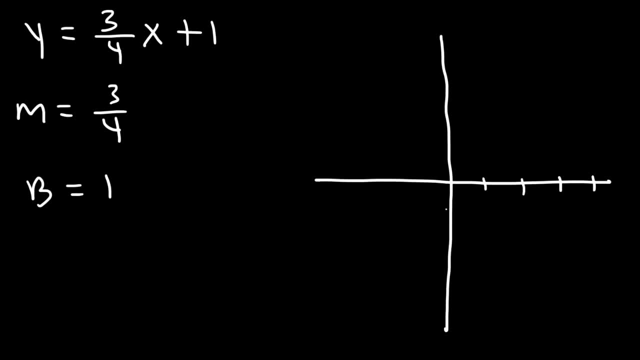 so, as always, the first thing we should do is plot the y-intercept, and so it's that positive one. it's above the x-axis this time, and the next thing we should do is use the slope to get the next point. so the slope is 3 over 4, so we 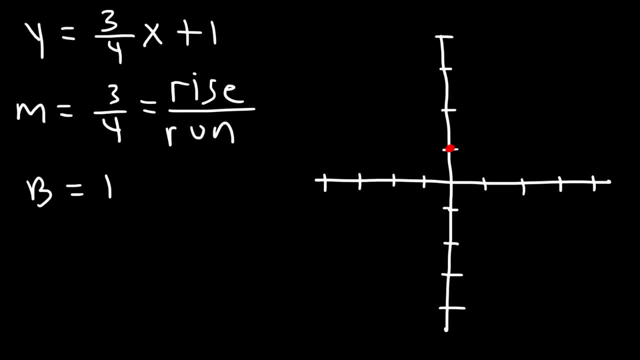 have a rise of 3 and a run of 4, so what this means is that we're going to go up three units and then we're going to travel four units to the right. so that will give us the point 4, comma 4, and then we could just connect. 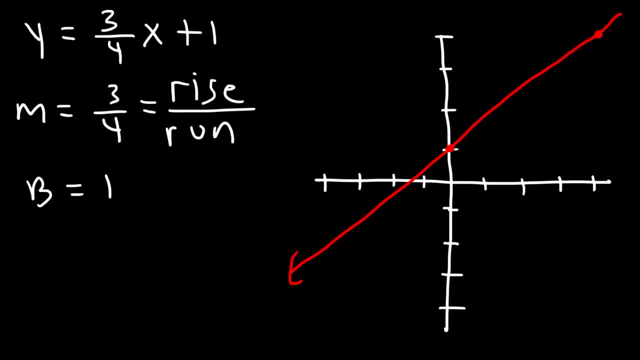 these two points with a straight line, and that's all we need to do for this example. so, as you can see, it's not too difficult to graph a linear function. now let's talk about how to graph linear equations. that is not in slope intercept form, but that is. 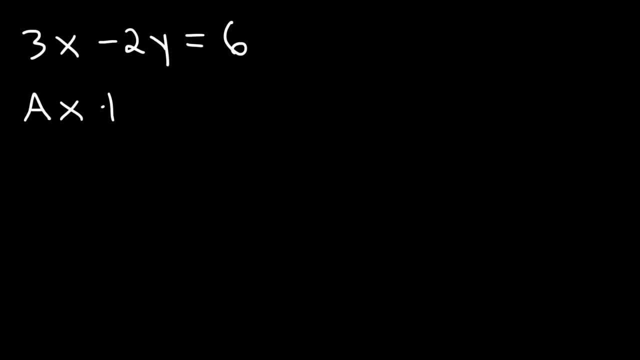 in standard form, that is, ax plus by, is equal to c form. so how do we do it in this case? one of the best ways to graph a linear function in this form is to find the x and the y-intercepts. to find the x-intercept. 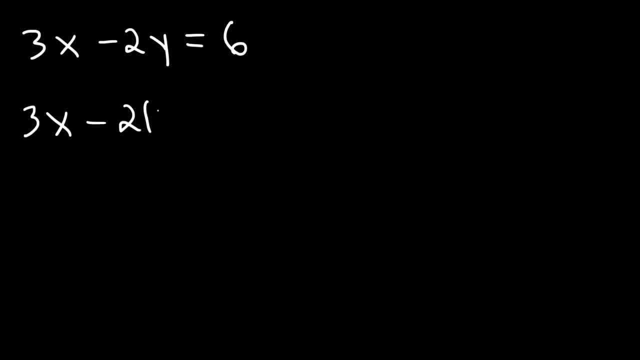 what you want to do is replace y with 0, and so 2 times 0 is 0. basically this disappears and you get 3. x is equal to 6 and our goal is to calculate the value of x. so if we divide both sides by 3, 6 divided by 3 is 2, so x is 2. this gives us: 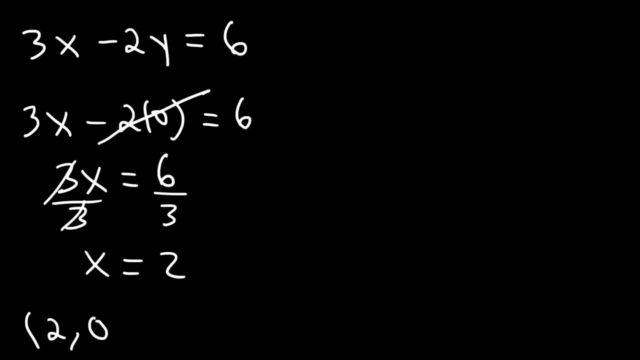 the x-intercept with an x- the value of 2 and a y value of 0, since we've replaced the y with 0. now to calculate the y-intercept, what we're going to do is replace x with 0 and calculate y. so 3 times 0, that disappears, that's just 0. 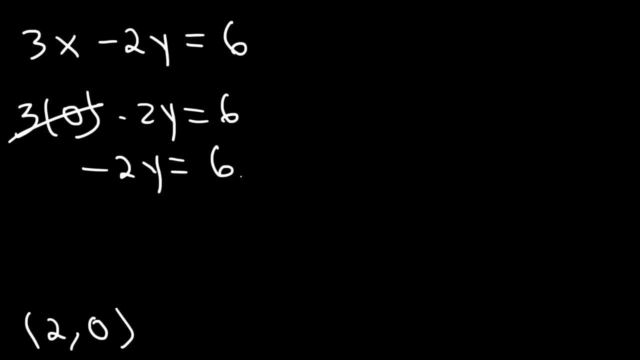 and so we have negative 2y is equal to 6 divided both sides by negative 2. we get that y is positive 6 divided by negative 2, which is negative 3. so we get the point 0, negative 3, and that is the y-intercept. now let's talk about 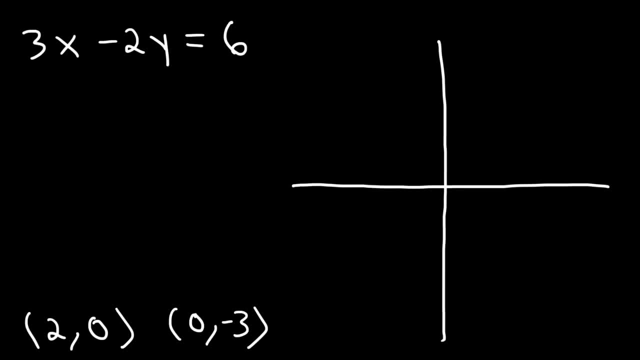 graphing this equation, so all we need to do is plot the x and the y-intercepts. that's it. so, starting with the x-intercept, it's at 2: 0, so x is 2, y is 0, and for the y-intercept, it's simply at negative, 3 along the y-axis. 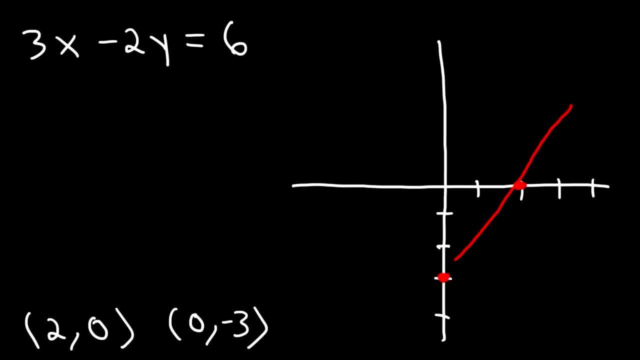 and now we just got to connect the two points with a line, and so that's how we can graph that particular equation. let's try one more example for the sake of practice. so go ahead and graph this equation: 2x plus 5y is equal to 10, so 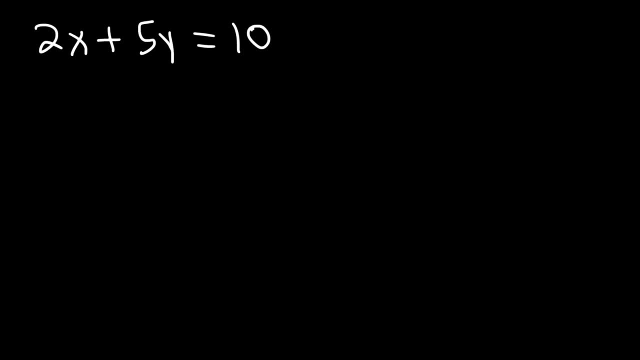 just like before, we're going to determine the x-intercept first. so let's replace y with 0. so 5 times 0 is 0, so we get the expression: 2x is equal to 10, and if we divide both sides by 2, 10 divided by 2 is 5, so the x-intercept is 5, given us.